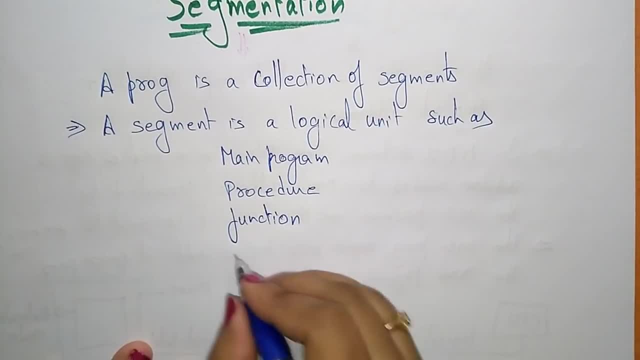 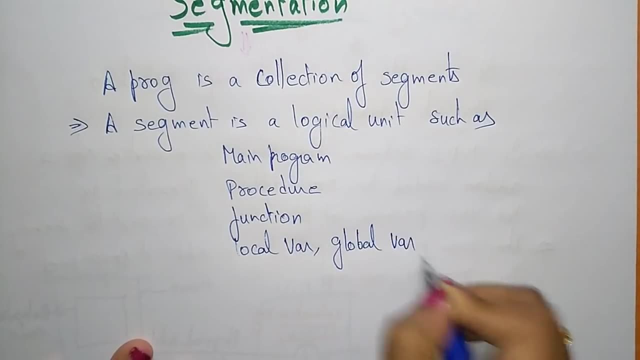 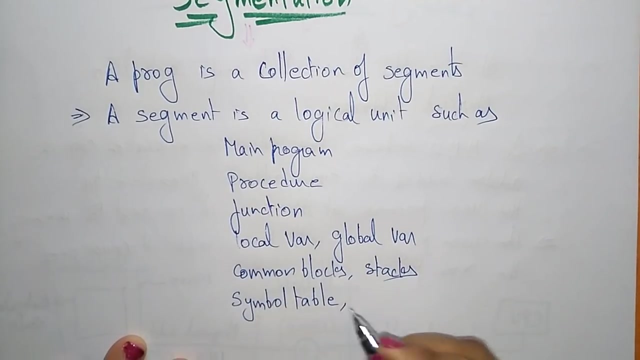 A program or outside the main program is also called as a segment or local variables. Local variables, global variables or common blocks or even stacks that are present in the program, or the symbol tables that we use in the program, or a process, or even arrays. So these are all called as a segments. 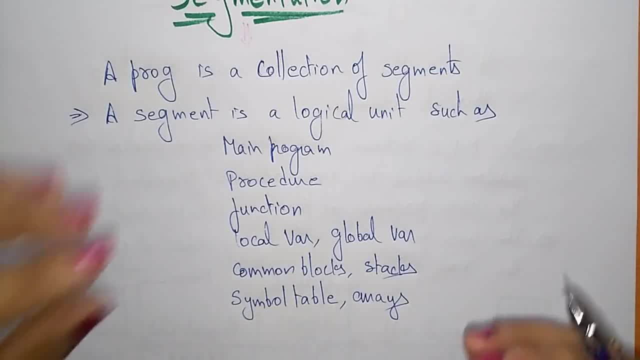 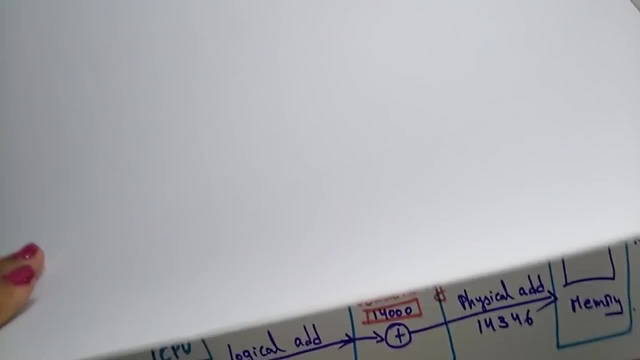 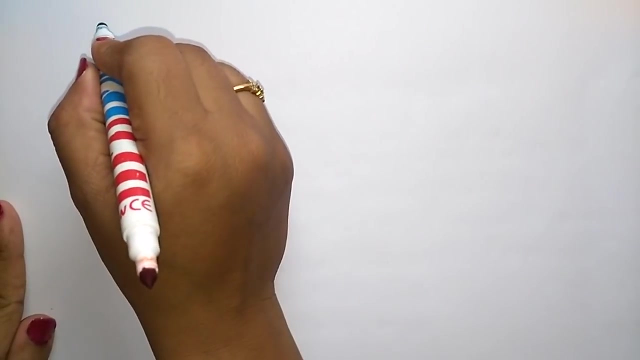 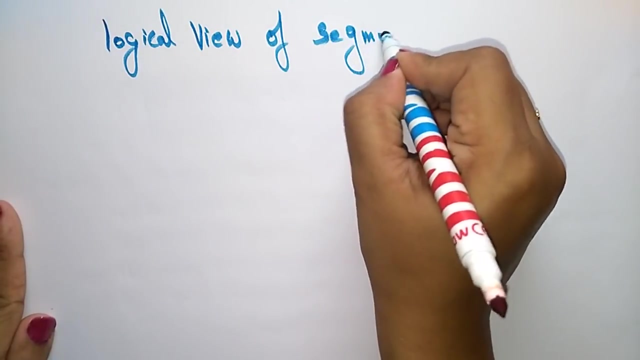 This. segments is nothing, but it is a logical unit consisting of all these modules. Now let us see the logical view of segmentation. So what exactly how? this logical view? I said the segmentation is a logical unit, So now let us see the logical view of segmentation. 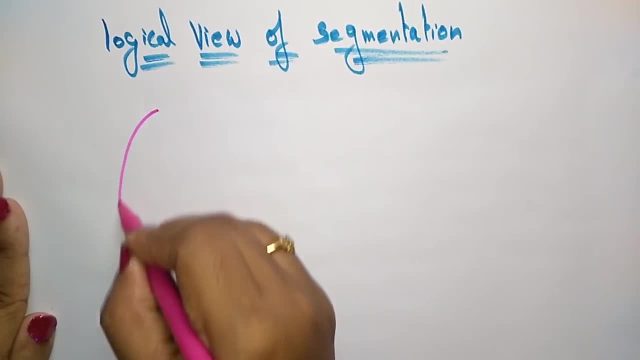 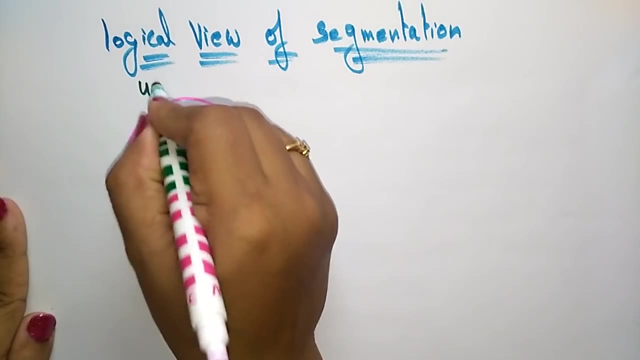 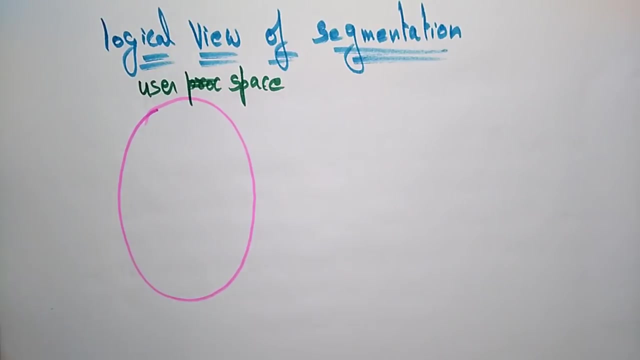 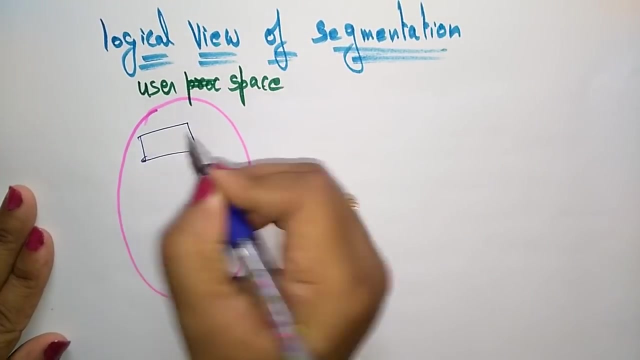 So let us take suppose this is, this is a user space. So user here, user is that is a user program User. let me write user space. Okay, So this user process is having a set of segments. So this is one segment. Let us take this is a subroutine of the program. 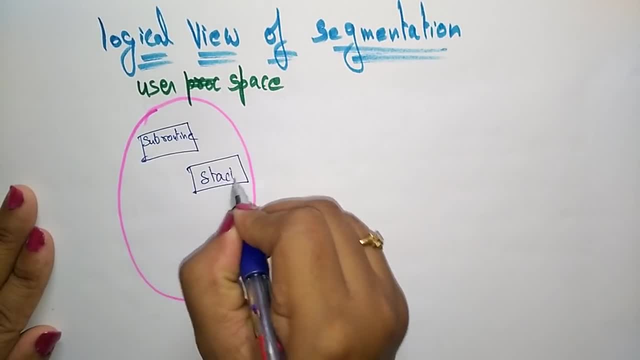 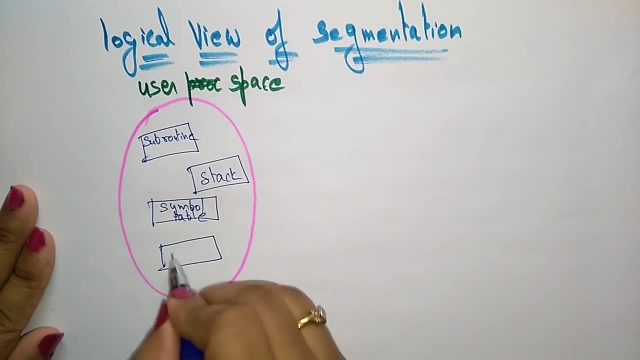 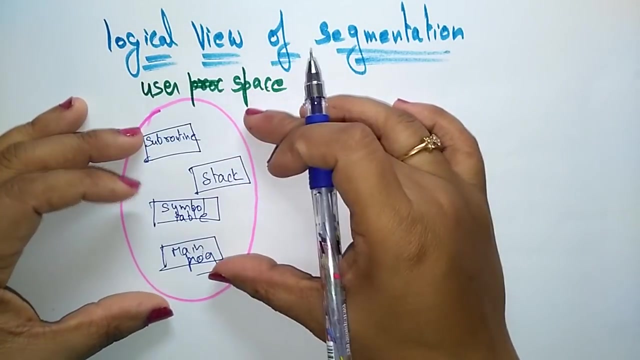 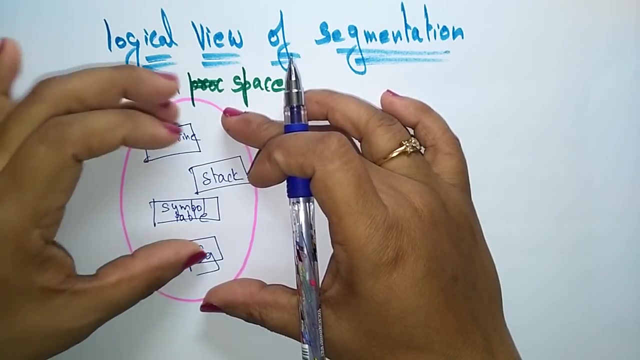 Okay, So this is a subroutine, And here suppose, let us take the stack, And here suppose, if you take the symbol table, And or else you can take the main program, So in this user space, the program, So here, whatever the user is giving the input, So that user is program consisting of set of segments. So this is a collection of a program, is a collection of segments, So this completely a program. This program is a collection of segments, So this is a 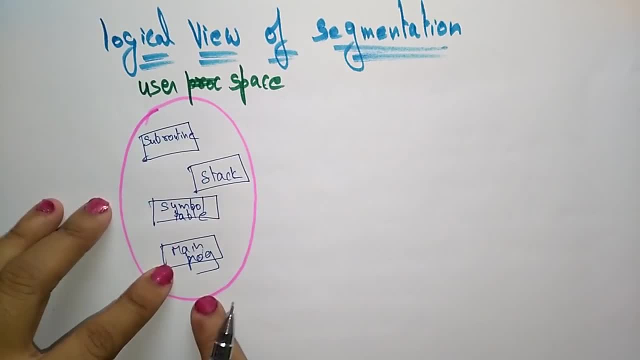 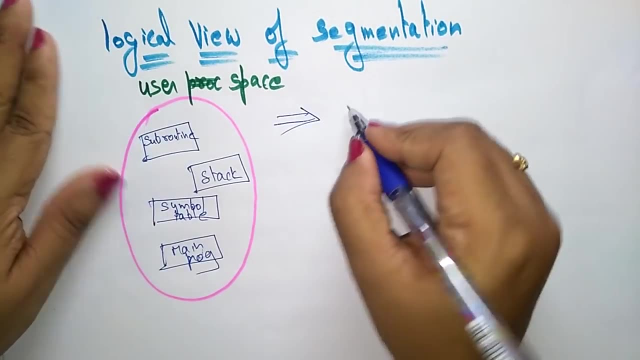 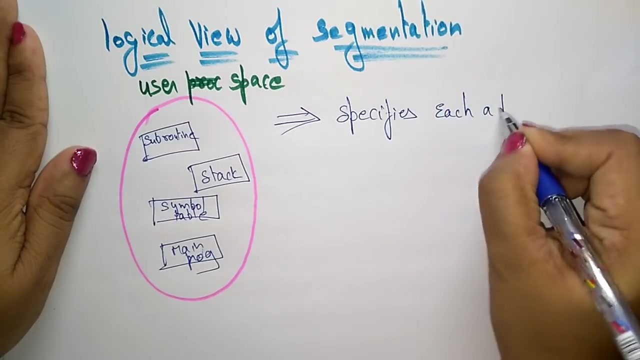 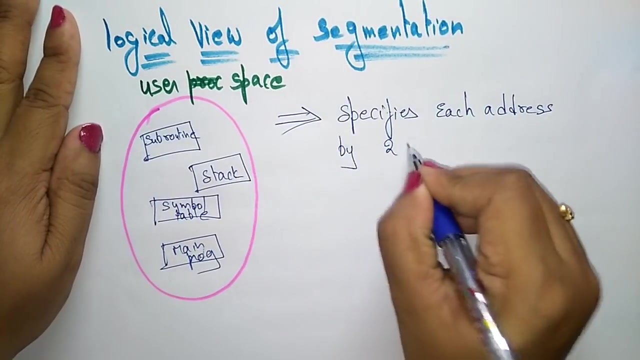 a segment, subroutine stack is one segment and symbol table and main memory. so here the user specifies each address by two quantifiers. the user always specifies, user specifies each address. so each segment is having some address right. so each address by two quantities. so what are those two quantities? so, with the help of segment name, 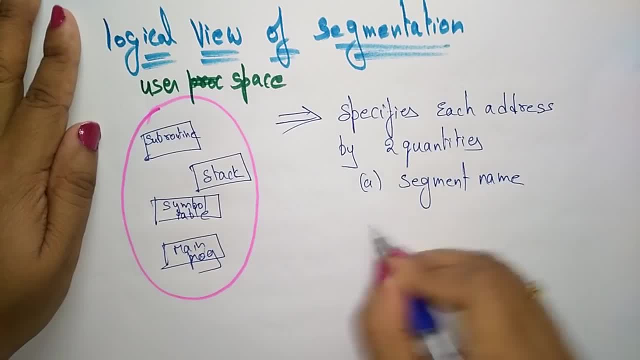 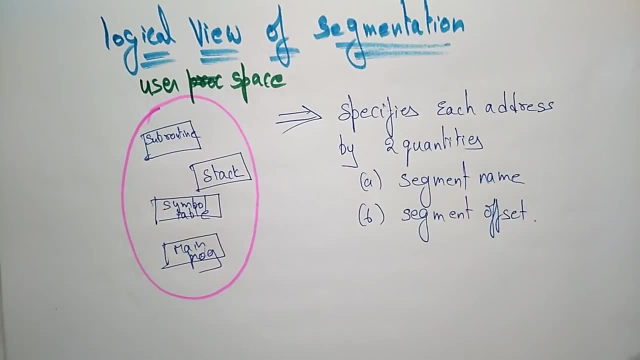 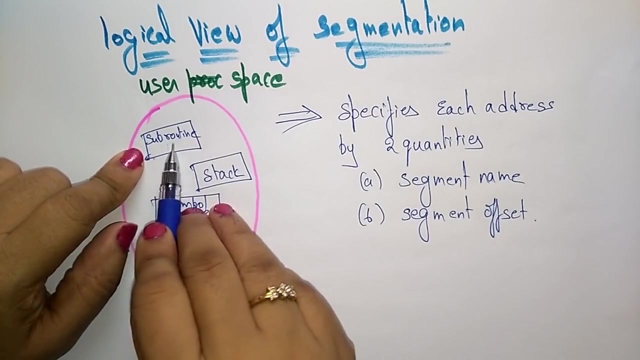 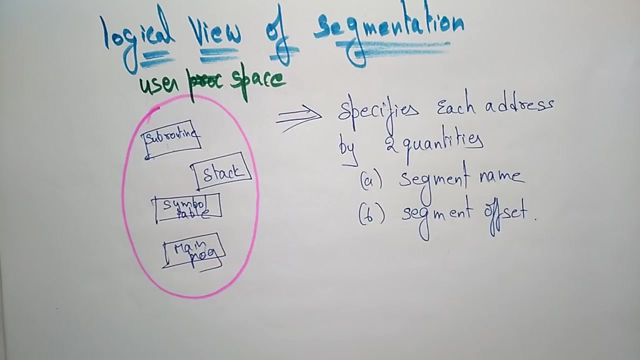 and segment offset. offset is nothing but it is the address. okay, so each address, so address of subroutine consisting of segment name, that is a subroutine, and the subroutine offset and stack name, stack name offset and symbol table, symbol table offset. so if you know that segment name and the offset, then the CPU can execute, can get the data in that particular address location. 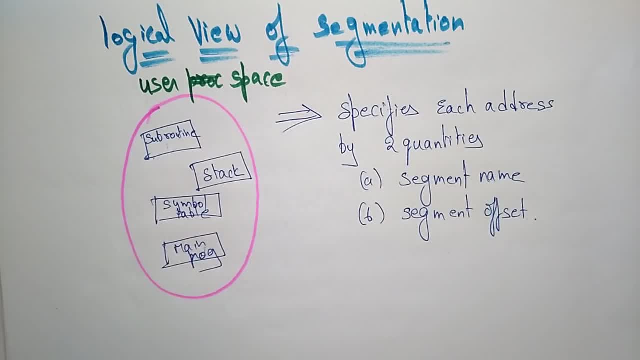 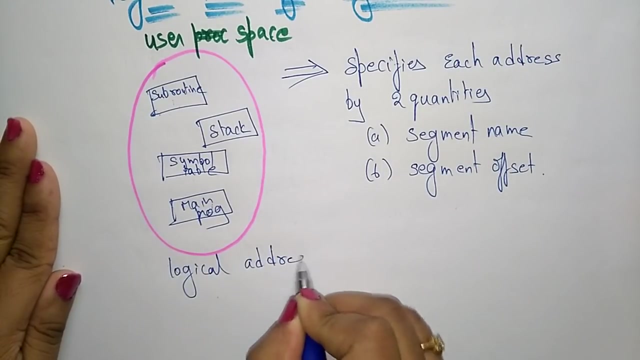 and execute the program so that everything is a logical view, okay, and whatever the result that you want to store in the main union memory unit. so that is the physical memory, physical space. so this is a logical address. so this is completely stored in logical address. so this logical address contains a tuples like 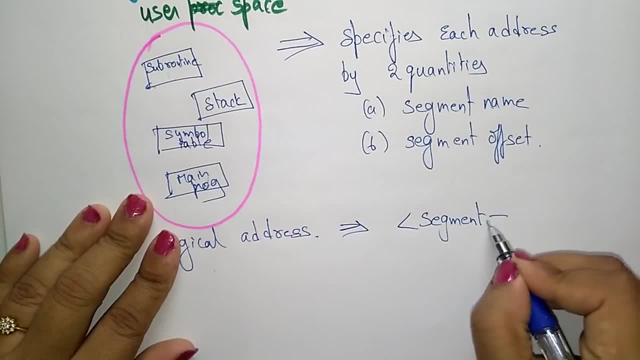 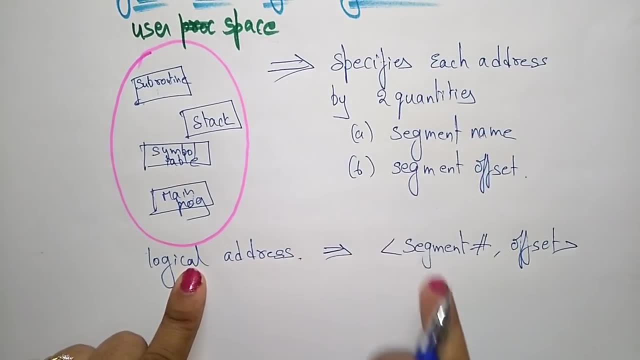 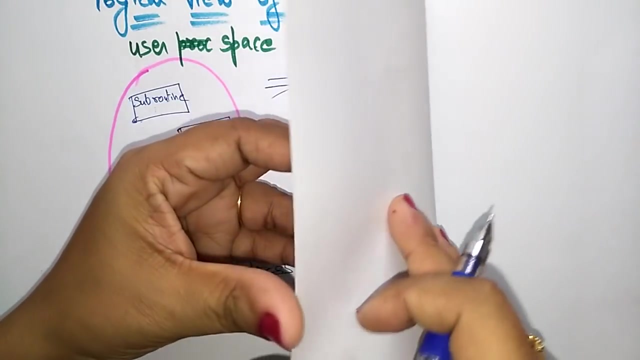 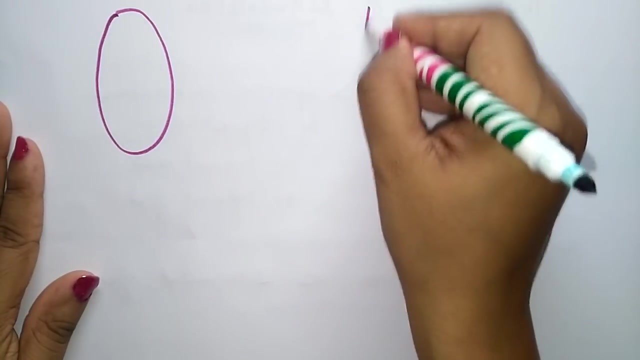 what it is: Segment, segment name and the offset. So the logical address consisting of this: two quantifiers, So that is a segment name and the offset. So let me explain with simple example. So just I am taking, suppose this is a user space and this is the physical. 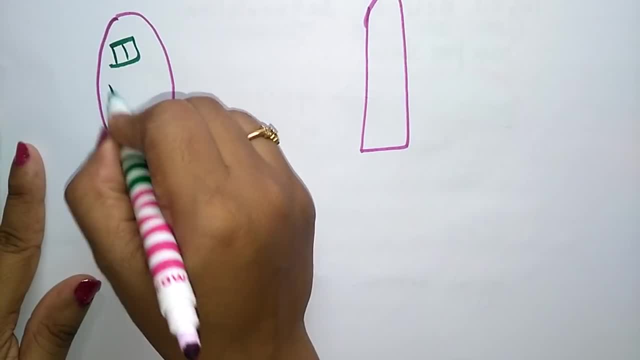 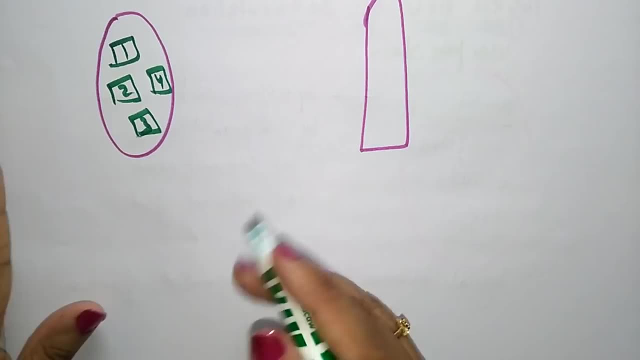 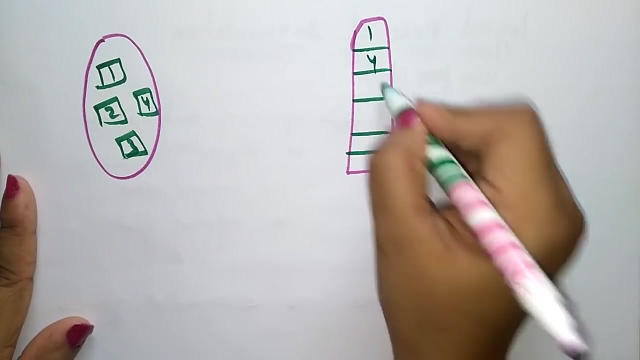 memory, So the user space, consisting of segments like 1,, 2,, 4,, 3.. So total they are having the four segments and here this is the memory unit, So 1, 4,, 2,, 3.. So this is a logical 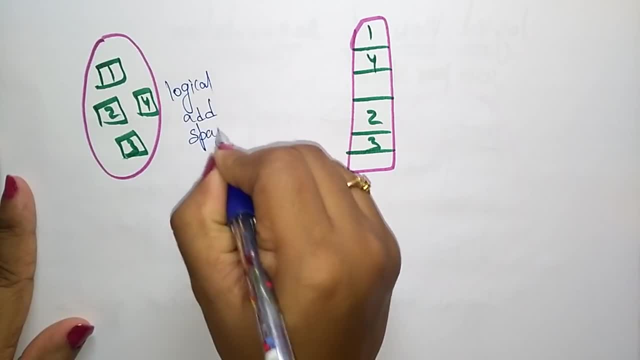 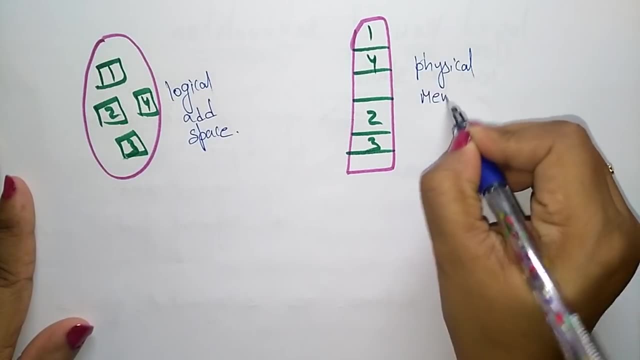 address this logical address space and this is the memory unit. So this is a logical address space and this is the memory unit. So this is the memory unit. So this is a. this is the physical memory space. So here, the logical address space, use the large programs. 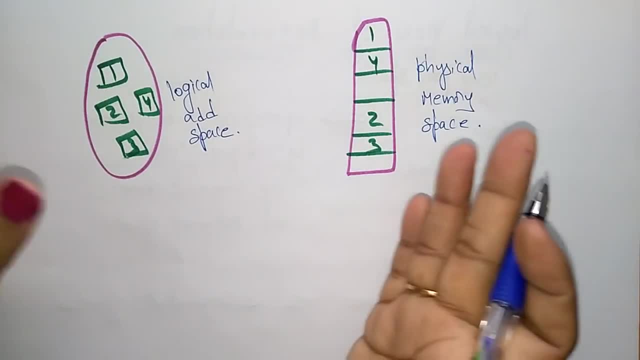 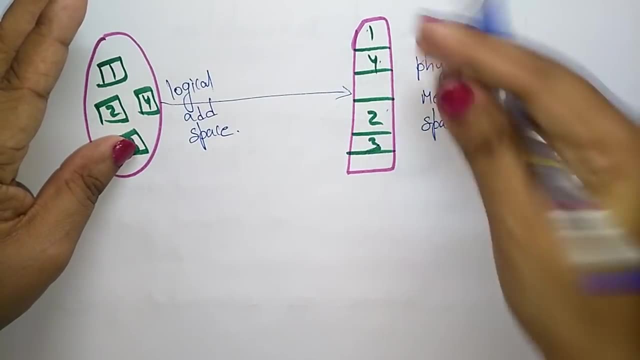 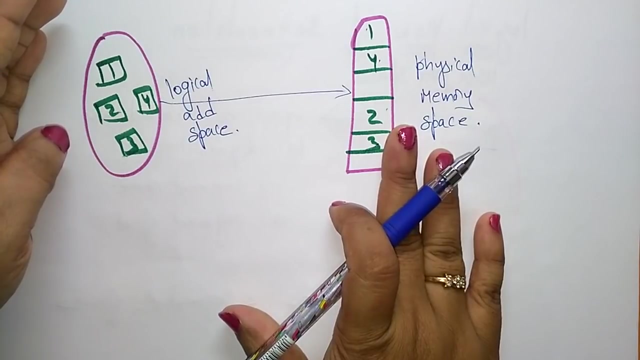 and these large programs will be converted, execute with the help of the CPU and stores in the physical memory space in the form of frames, So the physical memory consisting of frames, so those segments will be stored in the physical memory space. So in between this,